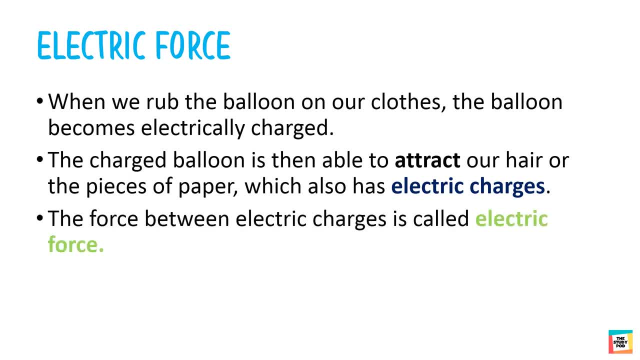 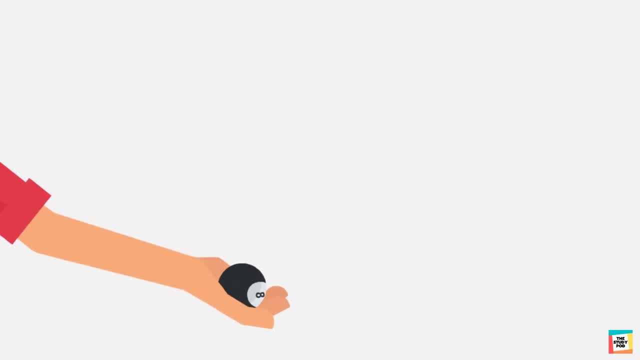 Rub the balloon near some parts of paper which also has electric charges. The force between electric charges is called electric force. Rub the balloon in the air. Does the balloon remain in the air or does it fall down? Why does the balloon fall down? 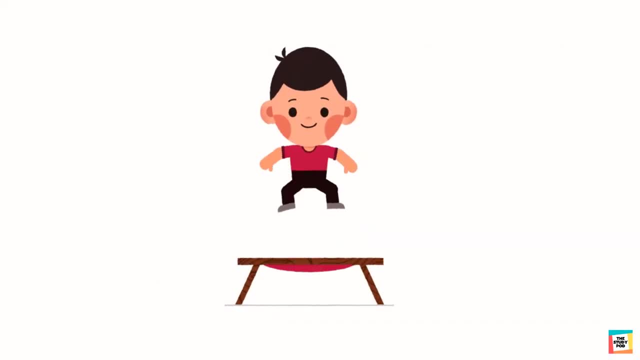 And why doesn't it remain in the air? No matter how high we jump, we will always land back on the ground. We do not stay up in the air. Why is that so? Let's find out. We land on the ground because there is a force pulling us down. 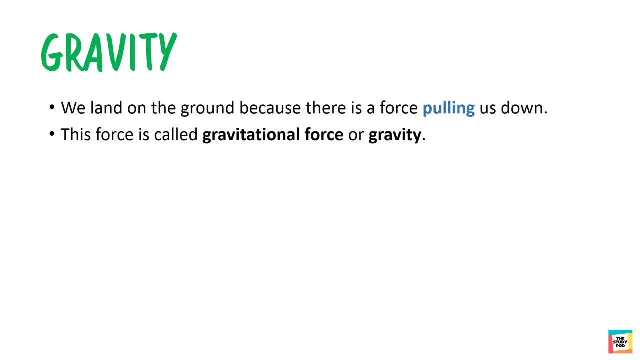 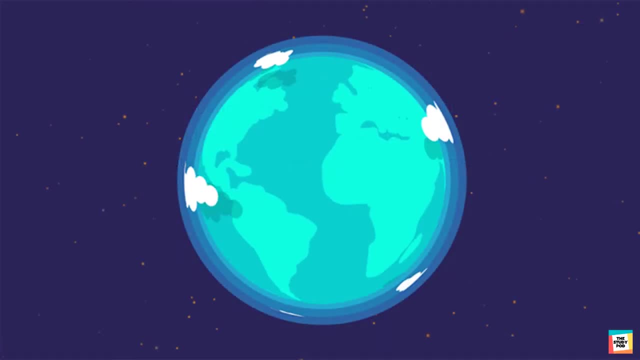 This force is called gravitational force or gravity. Gravity is the force of attraction between two objects. There is a force of attraction between the earth and any object near the surface of the earth. That is why objects in the air always fall back to the ground, towards the center of the earth. 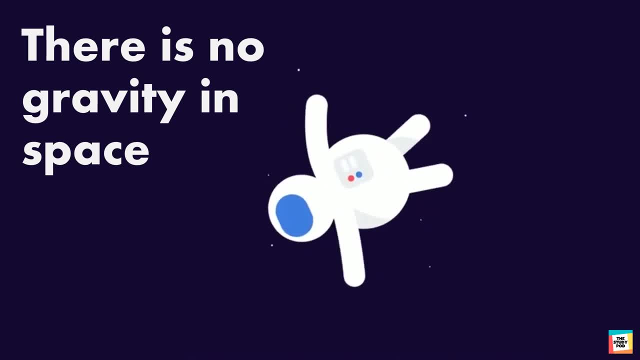 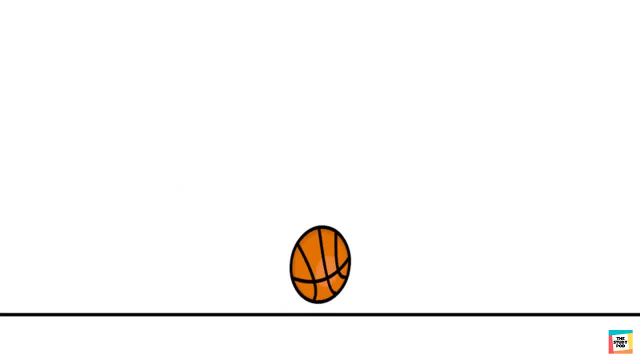 There is no gravity in space. This is why astronauts and other things float around in space. Toss a ball on the ground. After bouncing for some time, the ball will slow down and come to a stop. Why is that so? A force is acting on the ball as it moves. 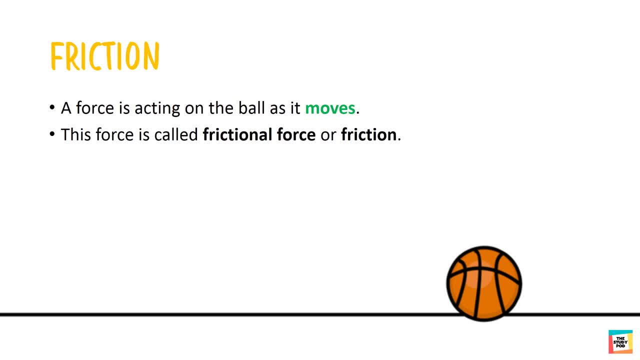 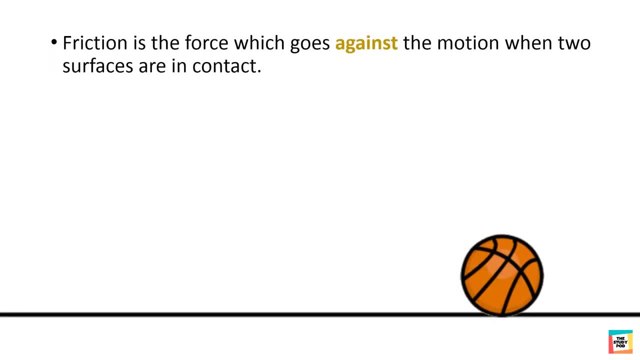 This force is called frictional force or friction. It makes the moving ball slow down and eventually stop. Friction is the force which goes against the motion. when two surfaces are in contact, It acts in the opposite direction to the motion. Friction is a contact force. 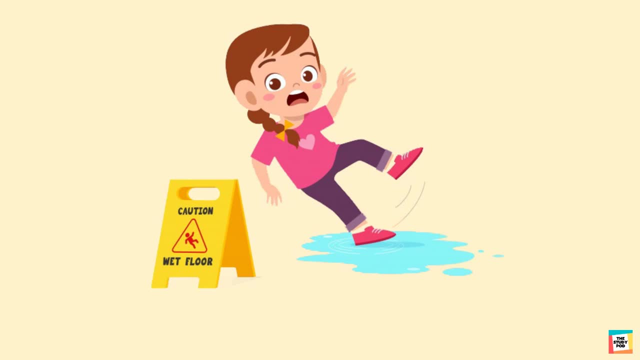 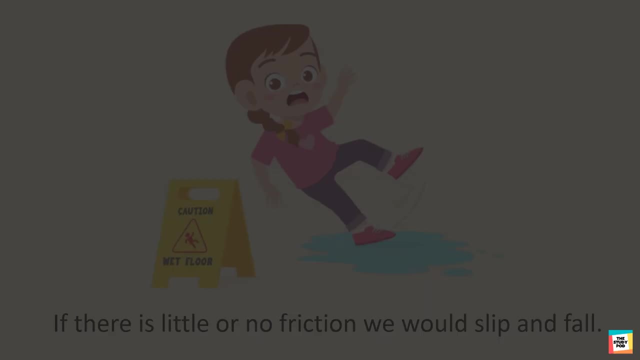 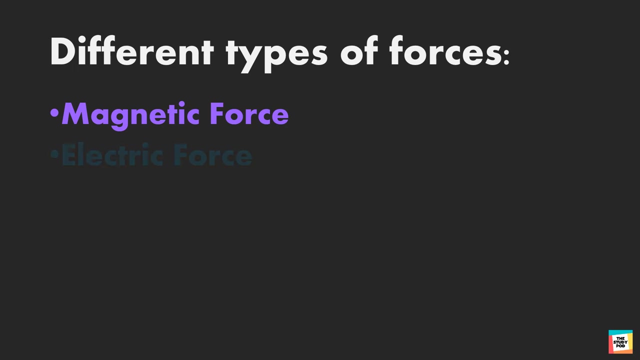 When we are walking, there is friction between our shoes and the ground. If there is little or no friction, we would slip and fall. So, kids, in this video we discussed different types of forces, Like the magnetic force, electric force, gravity and friction. 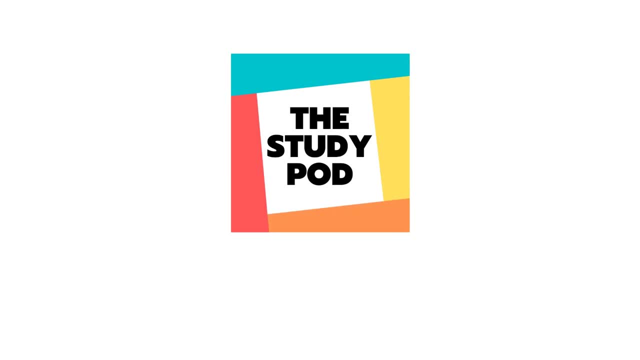 This brings us to the end of the video. If you have any queries, you can write to us at thestudypod01 at gmailcom.